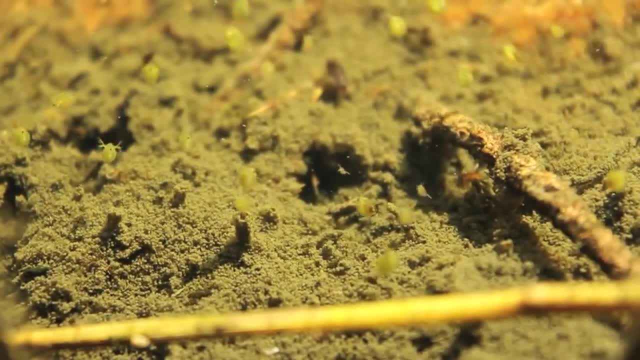 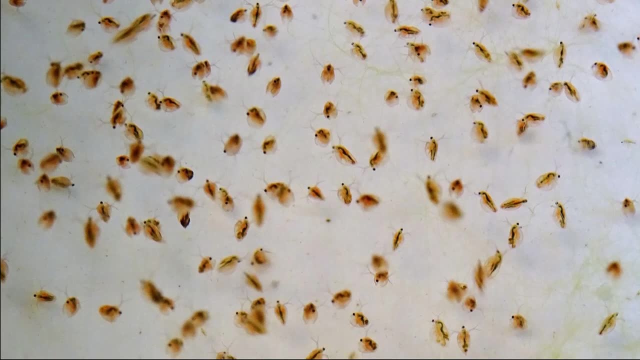 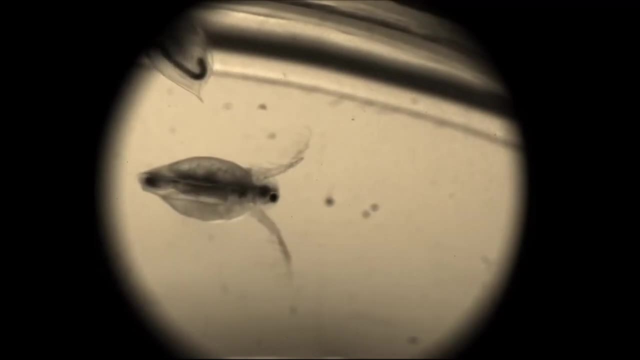 Common water fleas are aquatic open water crustaceans that are part of the zooplankton. They are found mostly in temperate freshwater lakes, but they can also tolerate brackish water. They are critical to lake health, providing food for fish and feeding on algae. 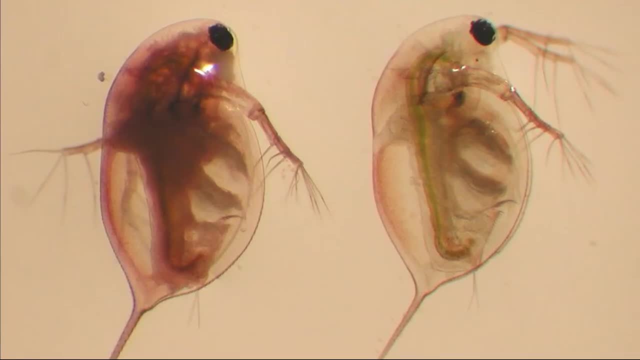 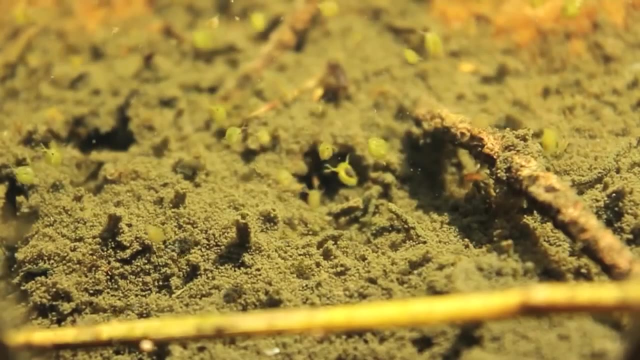 Water fleas are filter feeders. They direct small suspended particles into their mouth by a water current produced by their leaf-like legs. They have a jumpy mode of swimming caused by the beat of the large antennae that are used for swimming. 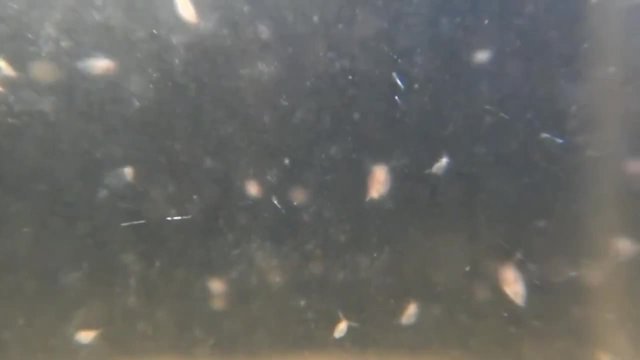 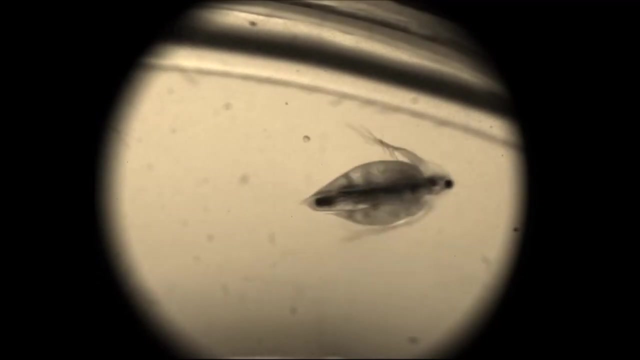 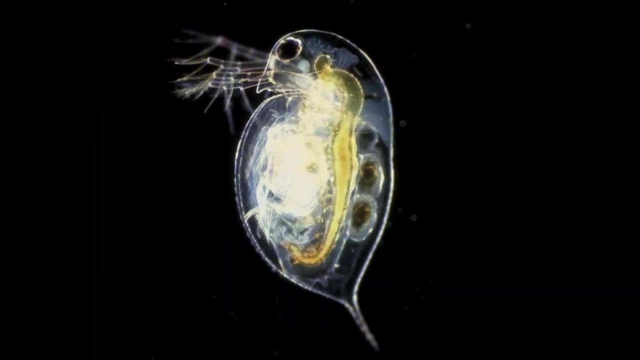 Swimming allows for travel between shallow and deeper waters. They retreat deeper during the day to avoid predation. They move closer to the surface at night, where food is abundant. A water flea's body is enclosed by an uncalcified shell. They have a simple heart. and an univocal brain. They have an immobilized body And makes it difficult to breathe. This is also simply harmful to the body. The body that we see in the video is probably not an oxytocin open circulatory system. 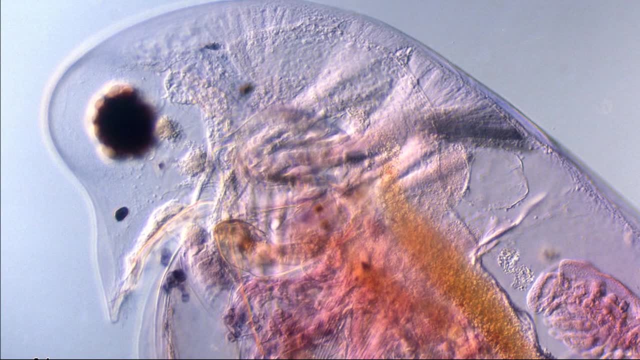 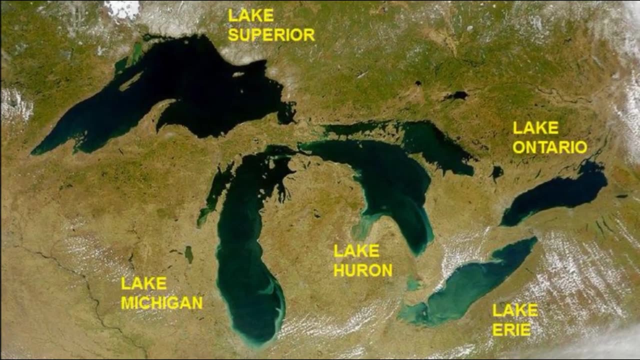 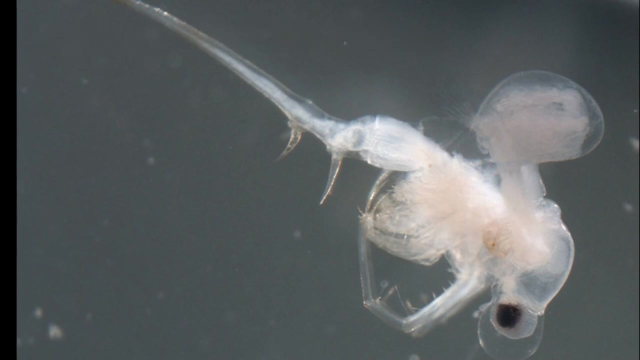 The head has a single large black eye. Their eyesight is poorly developed. Their numbers are declining in areas like the Great Lakes because of an invasive predator called the spiny water flea. Spiny water fleas are larger than common water fleas and they like to feed on them. 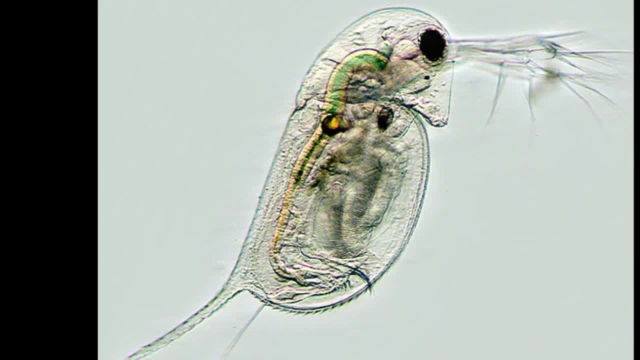 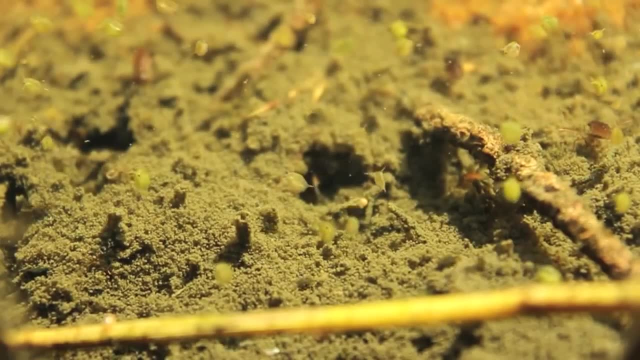 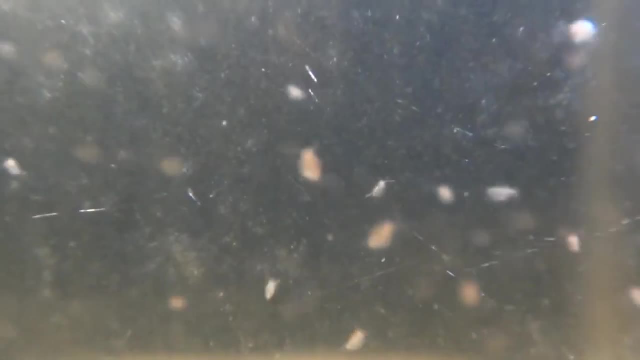 Common water fleas typically range in size from less than a millimeter to several millimeters long. Females are larger than males. Depending on environmental conditions, they may have both sexual and asexual life cycles. Females can reproduce asexually by parthenogenesis. 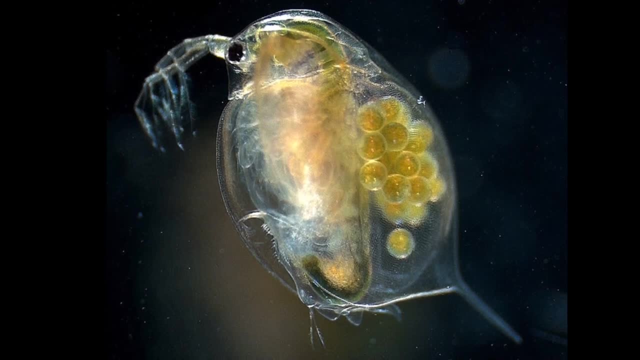 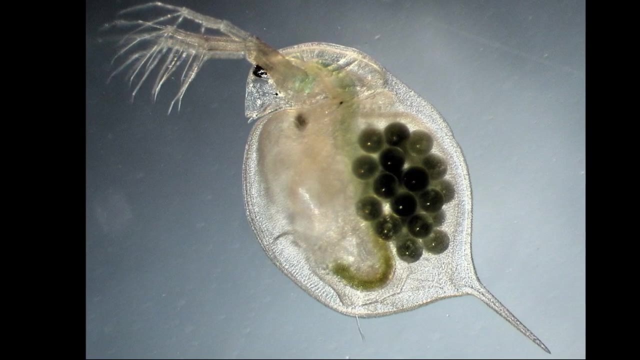 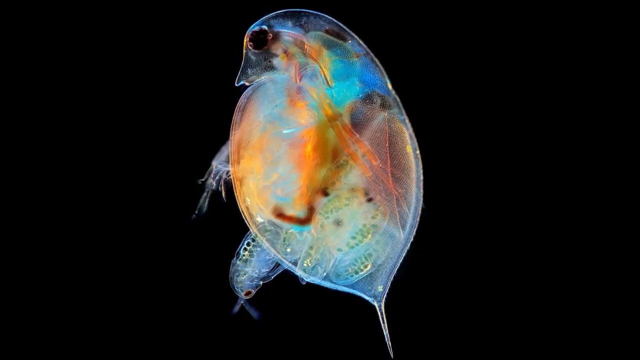 No mate needed. Typically, a female produces a clutch of parthenogenetic eggs. after every adult molt, The eggs are put in a brood chamber and start developing immediately. It may only take a day for the eggs to hatch. The hatched water fleas remain in the brood chamber for about three more days before being. 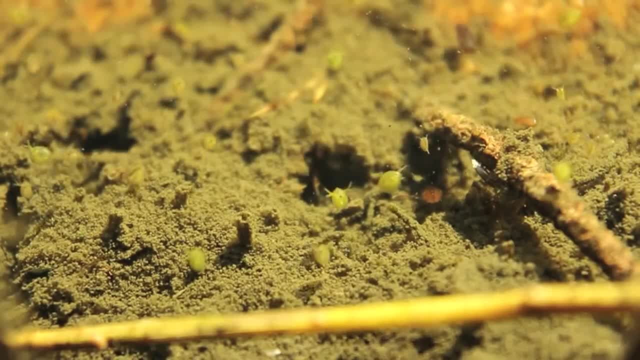 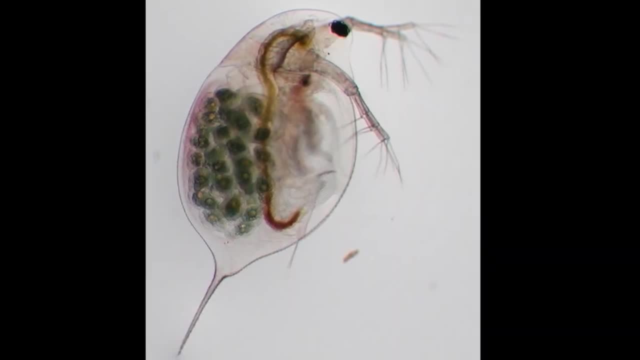 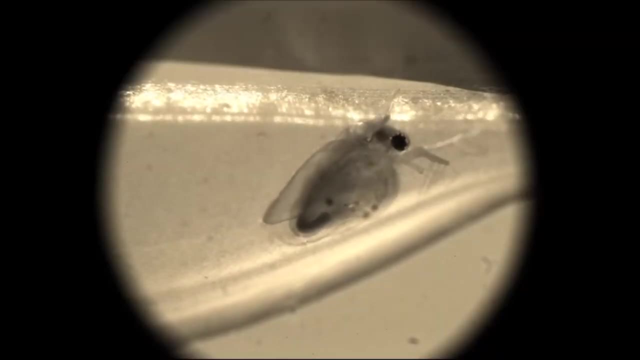 released. Females live around two months and they may produce a clutch of eggs every three to four days until death. Clutch sizes vary greatly by species, from only a few eggs to more than 100.. A different type of egg is produced for sexual reproduction.